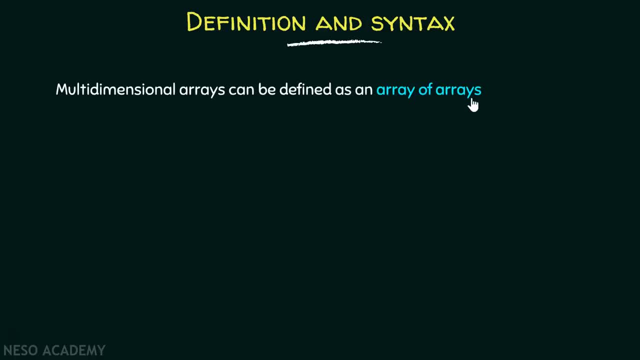 Multidimensional arrays can be defined as an array of arrays. You can think of multidimensional arrays as the combination of multiple arrays. Okay, Apart from this, the general form of declaring n-dimensional arrays is as follows: You have to specify the data type. 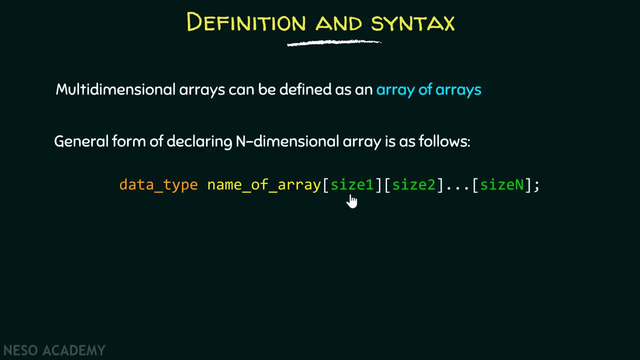 then the name of the array and then these square brackets, And inside these square brackets you have to put these sizes, That is, the number of elements. Like, for example, suppose I want to declare a two-dimensional array, then it should look like this: 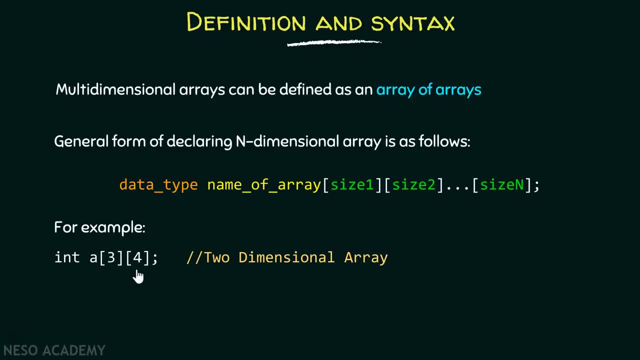 You have to specify the data type, the name and these sizes. Okay, If you want to declare a three-dimensional array, then it should look like this, And for four-dimensional array, you have to specify one more size. Okay, I will discuss in details about them. 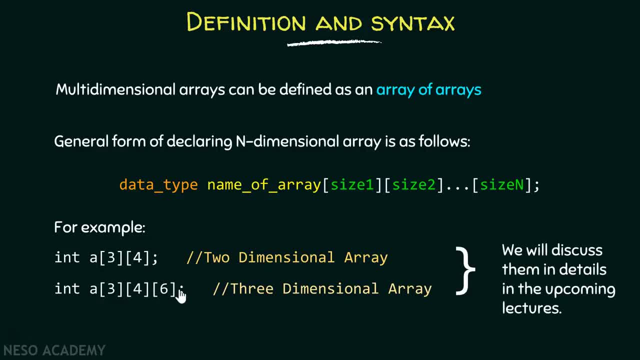 in the upcoming lectures, Like what is two-dimensional array and what is three-dimensional array. Okay, I will discuss them in the upcoming lectures. After defining the multidimensional array and giving the syntax, let's now try to understand how we can calculate the size of multidimensional arrays. 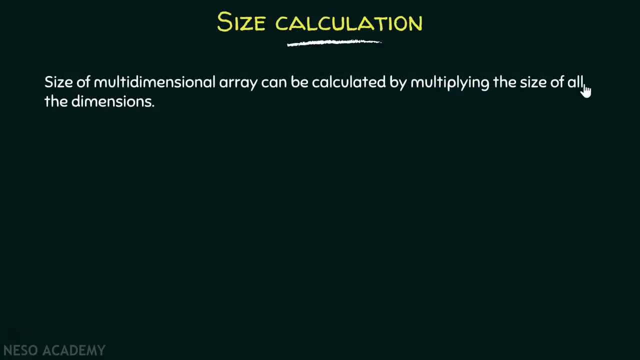 Size of multidimensional array can be calculated by multiplying the size of all the dimensions. You can calculate the size of multidimensional array by multiplying the size of all the dimensions, Like, for example: suppose I want to calculate the size of this particular array. 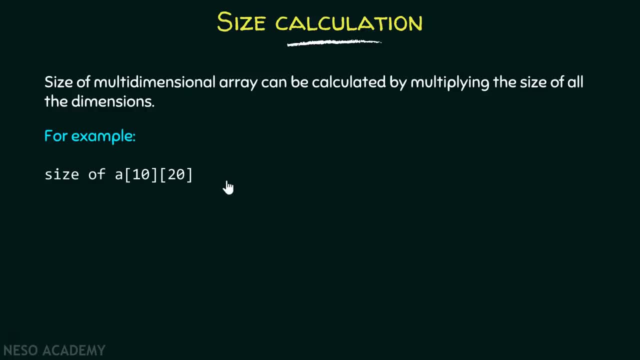 then I just have to multiply these two sizes. that is the number of elements. It gives me two hundred, which is the total number of elements it can contain. Right, But I want to know the size in bytes. Then I have to multiply two hundred by four. 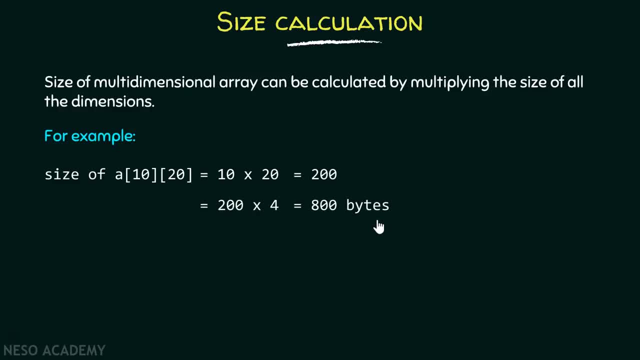 Okay, And it gives me eight hundred bytes. But wait, what is this four? Four means the size of one element. Four here depicts the size of one element. Okay, So that is why I am specifying four here And multiplying four by the total number of elements. 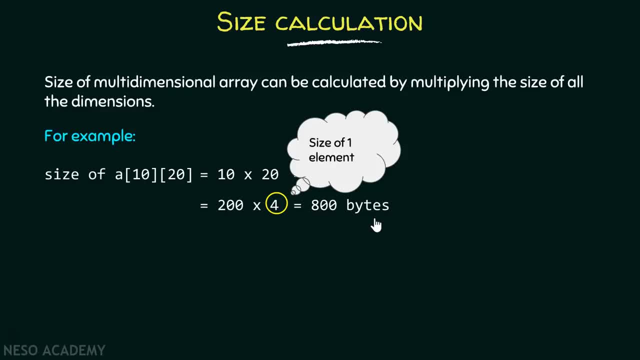 gives me the total size, which is eight hundred bytes. Now suppose I want to calculate the size of this particular array. then I have to multiply all these three sizes And it gives me the total number of elements. Here size means the number of elements.